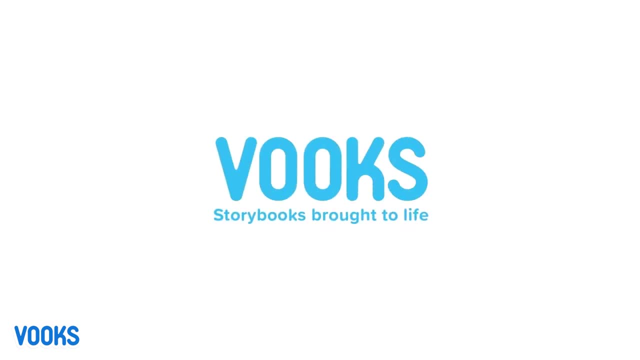 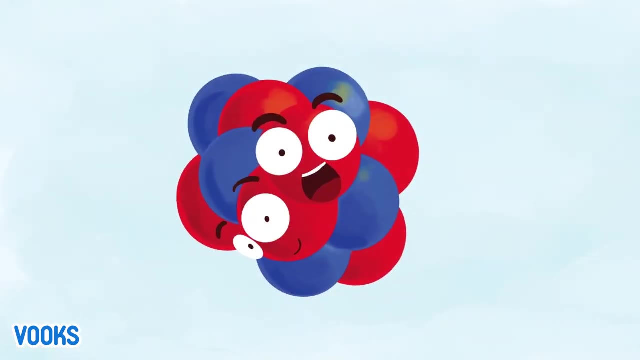 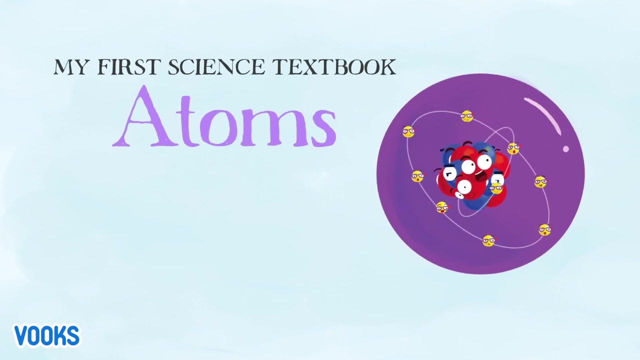 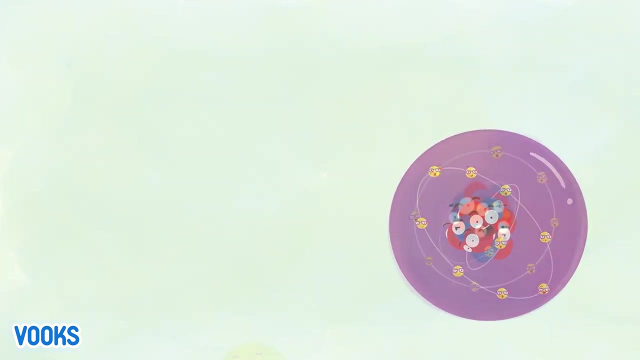 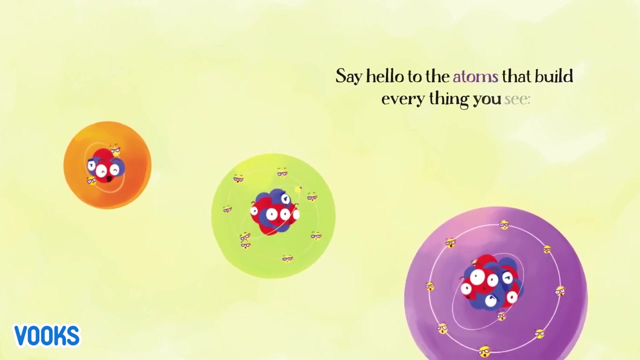 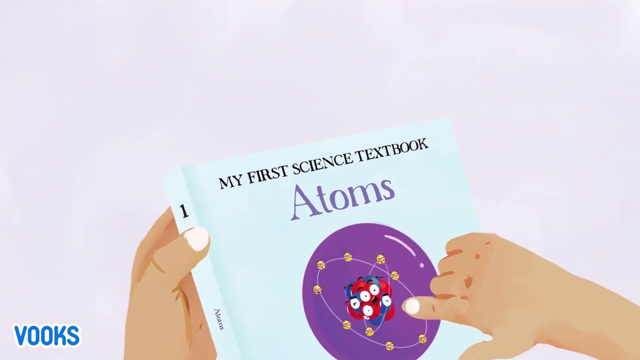 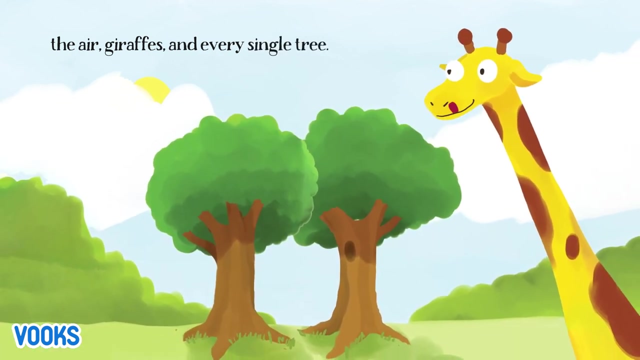 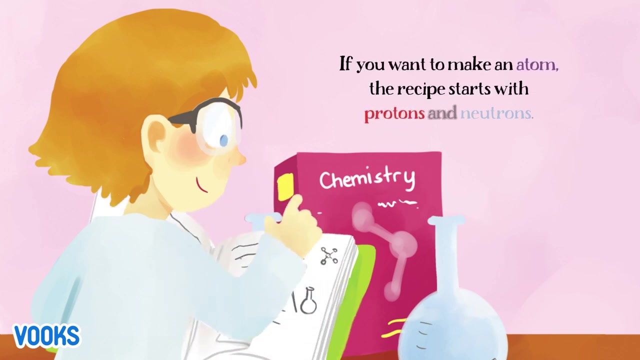 My first science textbook: Atoms. Say hello to the atoms, Atoms that build everything. you see, Your hands, this book, the air giraffes and every single tree. If you want to make an atom, the recipe starts with protons and neutrons. 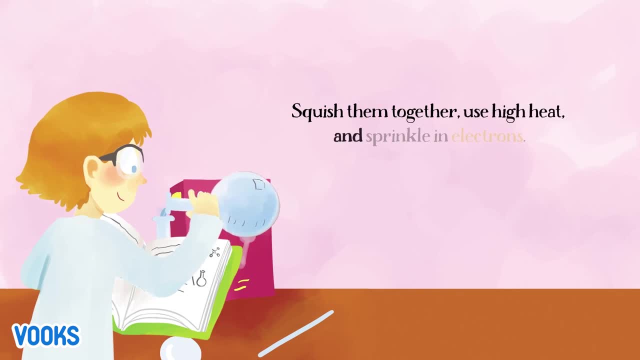 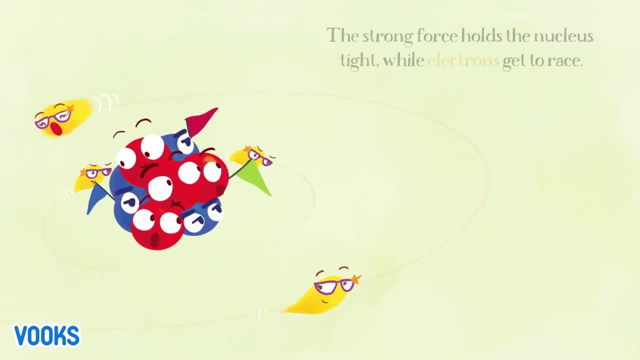 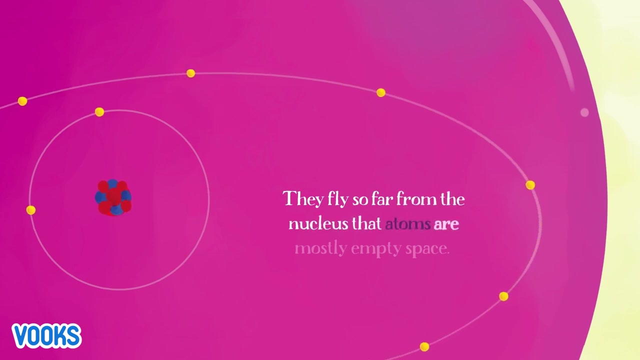 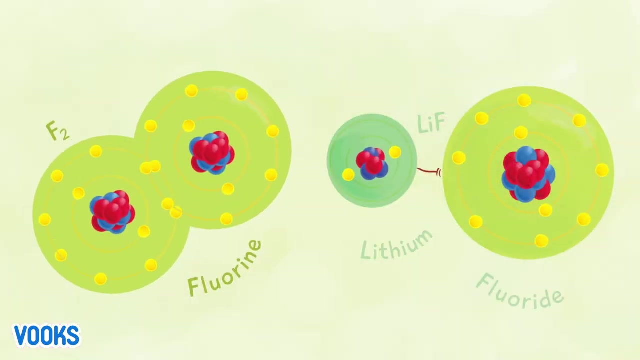 Squish them together, Use high heat and sprinkle in electrons. The strong force holds the nucleus tight, while electrons get to race. They fly so far from the nucleus that atoms are mostly empty space. Fluorine, Fluorine, Lithium. 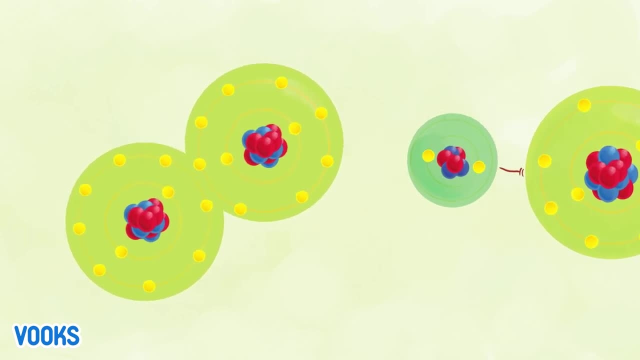 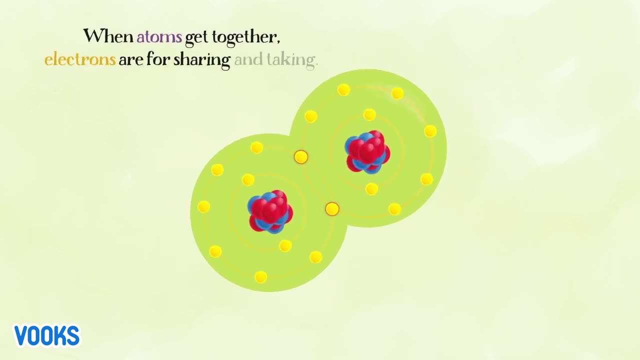 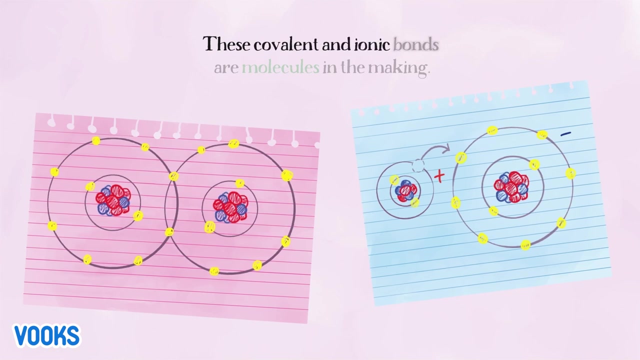 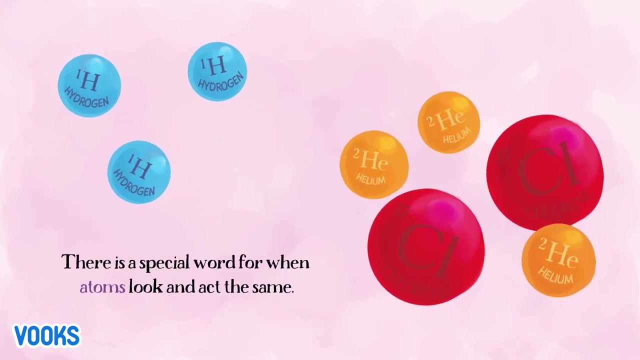 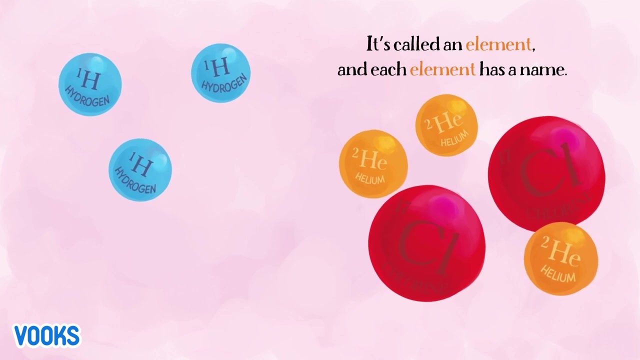 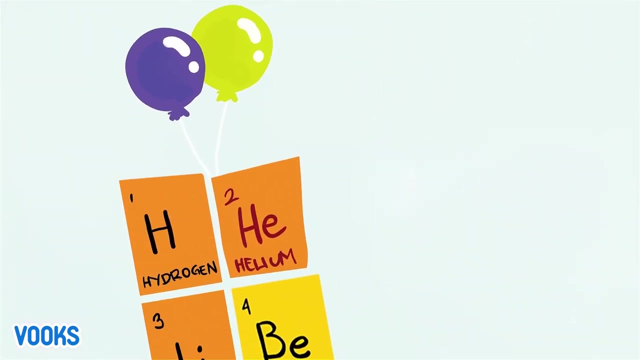 Fluoride. When atoms get together. electrons are for sharing and taking. These covalent and ionic bonds are molecules in the making. Covalent bond: Ionic bond: To take an atom. it include nelon, hydrogen and hydrogen. 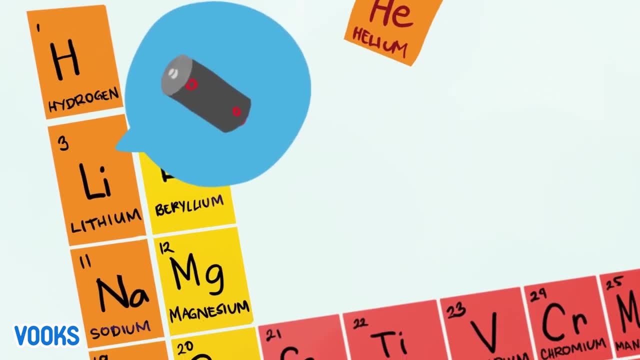 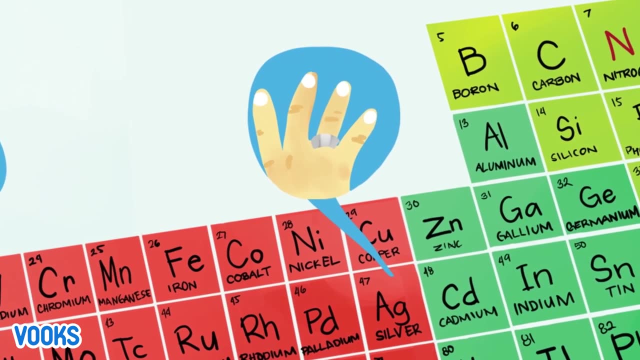 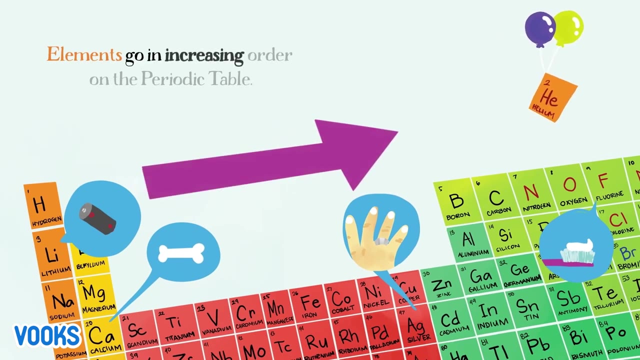 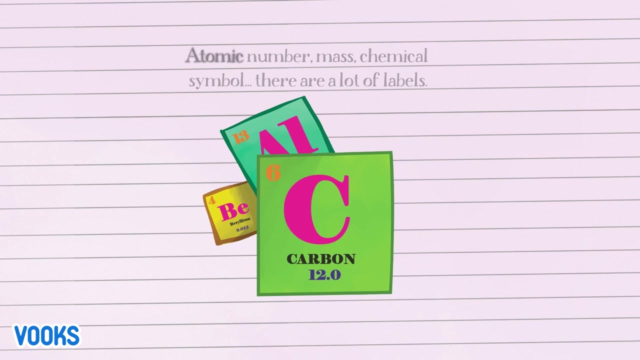 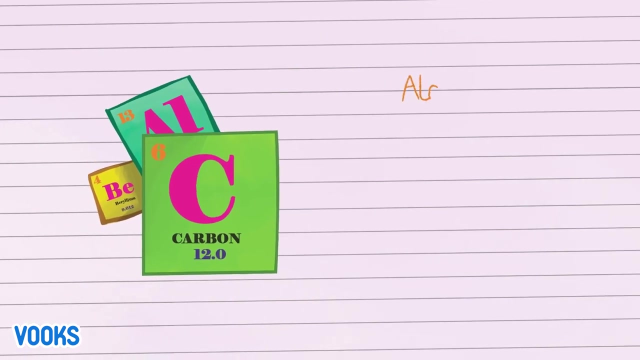 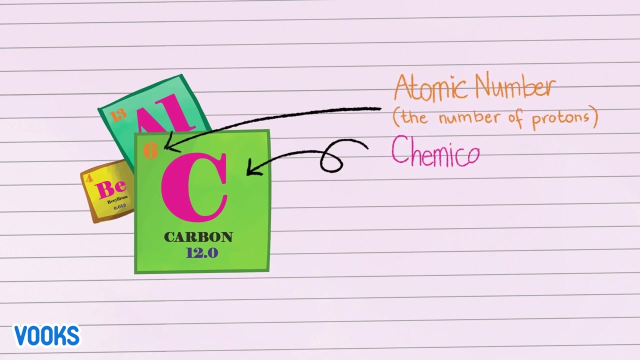 Carbon, Not iron. three calcium, 20, silver, 47, fluorine. nine elements go in increasing order on the periodic table. atomic number, mass, chemical symbol. there are a lot of labels here. atomic number: the number of protons. chemical symbol name: atomic mass: the number of protons and neutrons. 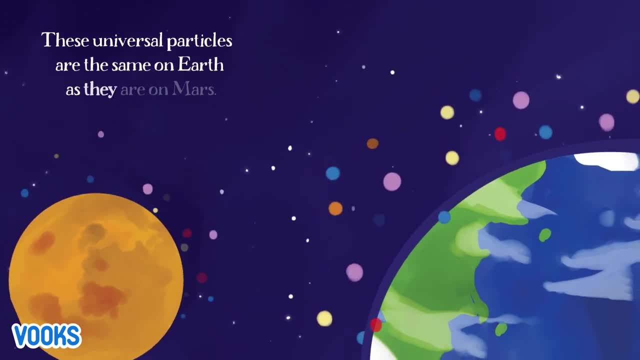 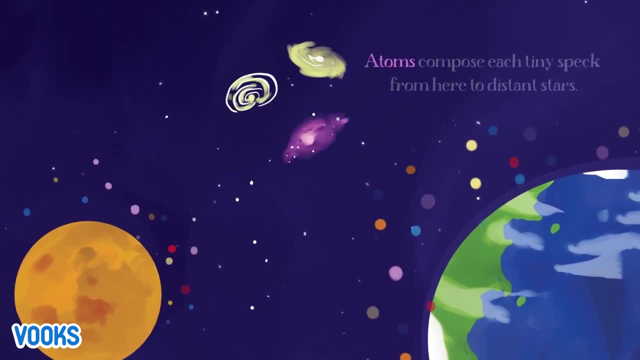 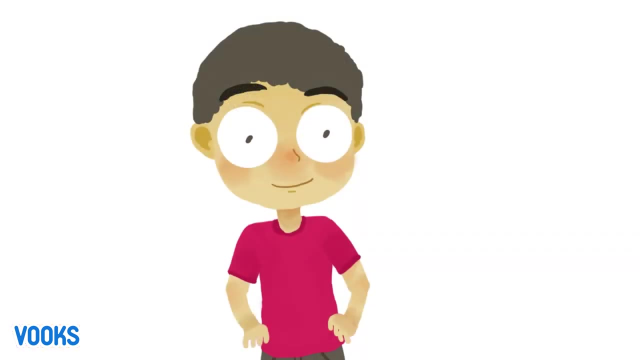 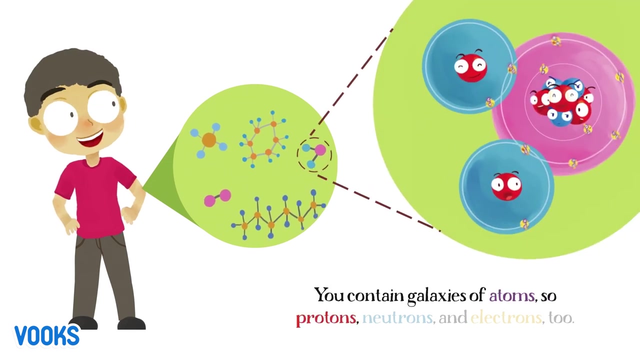 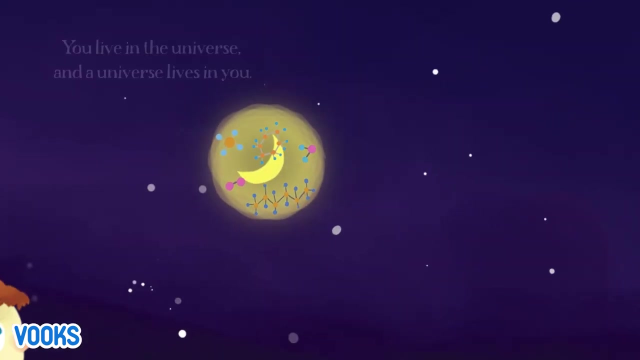 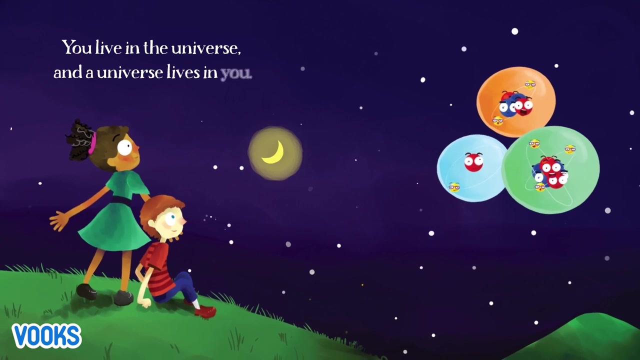 these universal particles are the same on earth as they are on mars. atoms compose each tiny speck from here to distant stars. You contain galaxies of atoms, so protons, neutrons and electrons too. You live in the universe and a universe lives in you. 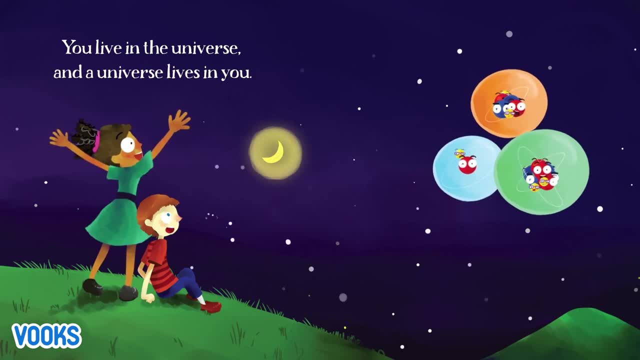 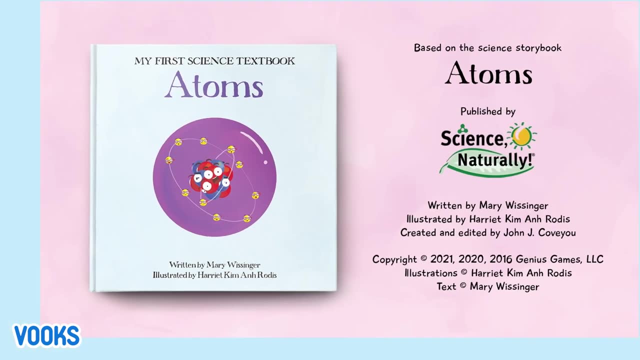 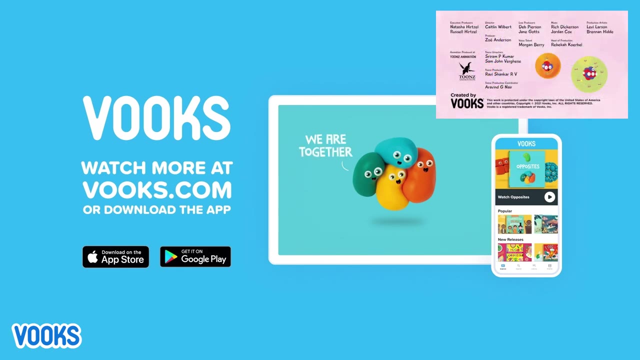 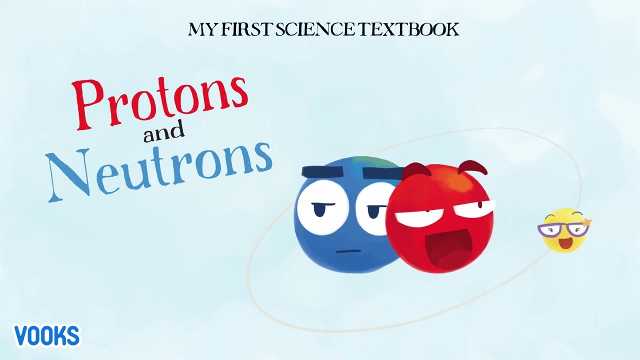 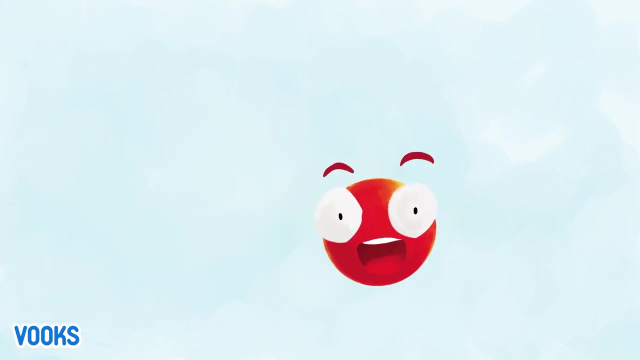 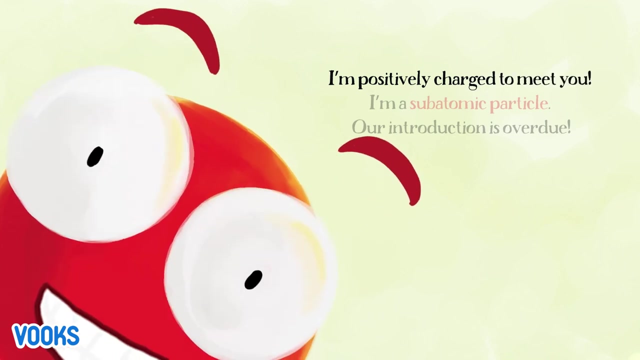 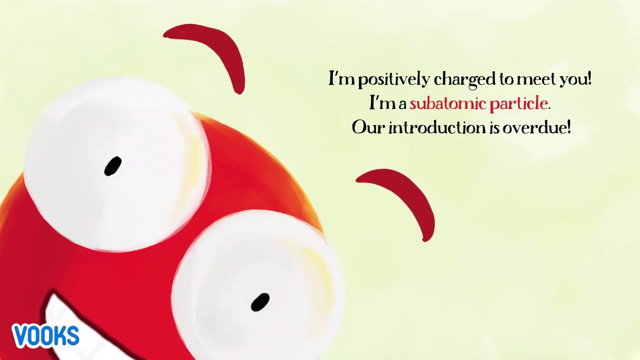 Join us at bookscom or download the app. My first science textbook: Protons and neutrons. I'm Pete the Proton. I'm positively charged to meet you. I'm a subatomic particle. Our introduction is overdue. I'm Pete the Proton. 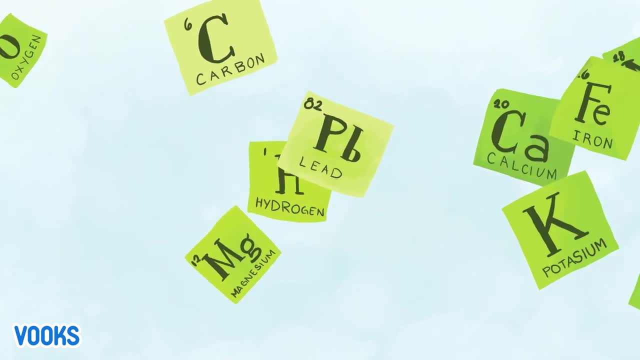 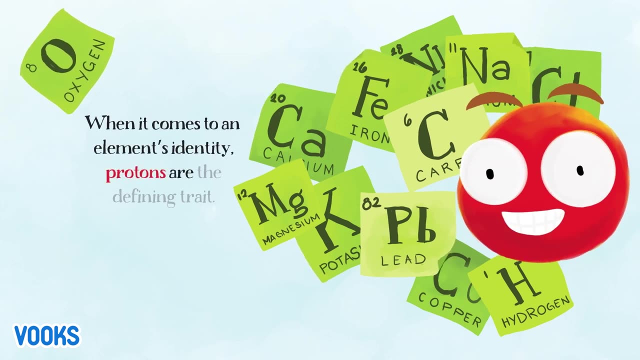 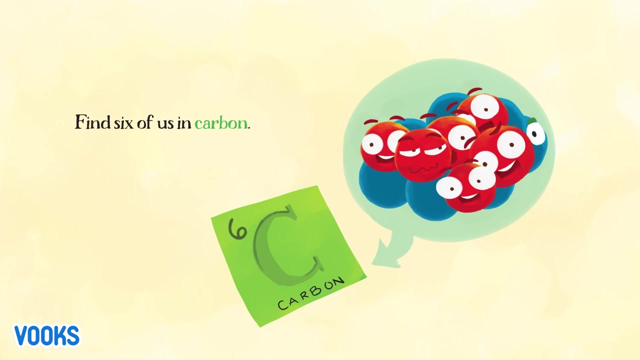 I'm positively charged to meet you. I'm a subatomic particle. I'm a subatomic particle When it comes to an element's identity. protons are the defining trait. Find six of us in carbon. In oxygen. find A. 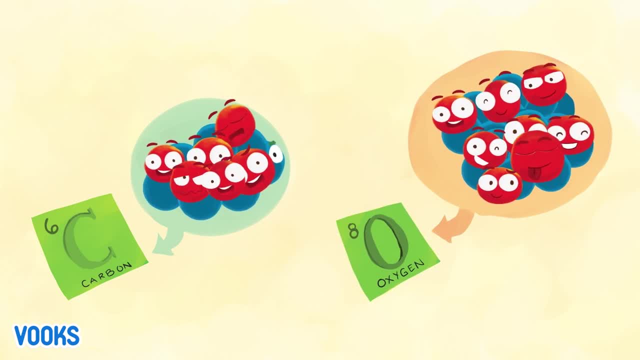 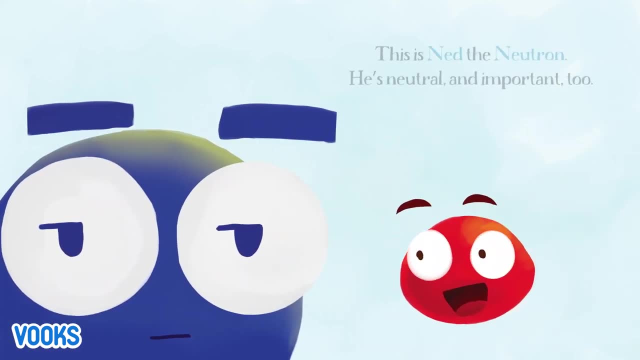 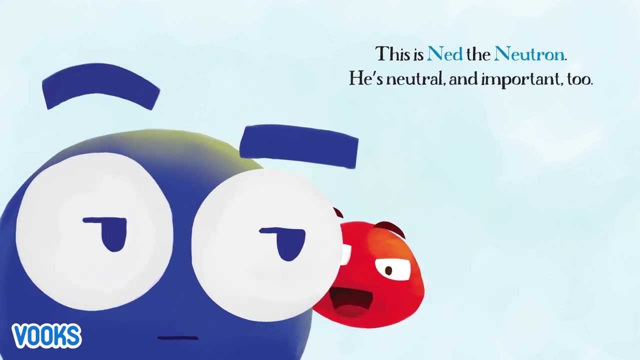 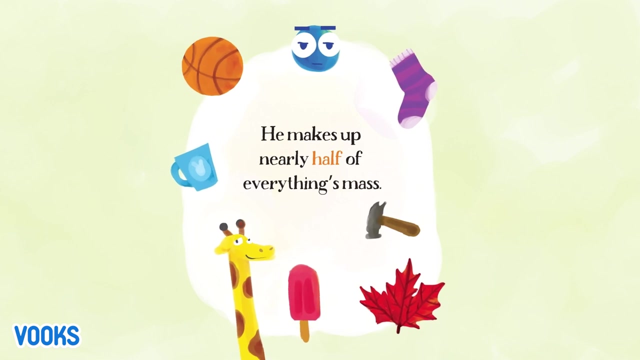 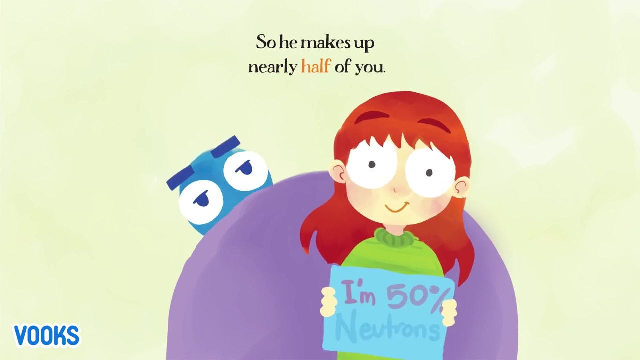 C, carbon, O oxygen, O oxygen. This is Ned the Neutron. He's neutral and important too. He makes up nearly half of everything's mass, So he makes up nearly half of you. I'm 50% neutrons. 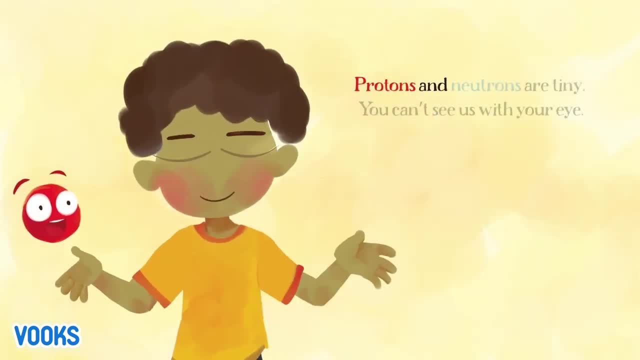 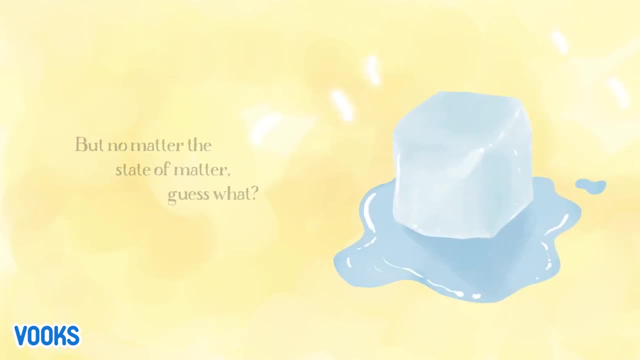 I'm 50% neutrons. I'm 50% neutrons. Protons and neutrons are tiny, You can't see us with your eye. But no matter the state of matter, guess what You'll find: me and this guy. 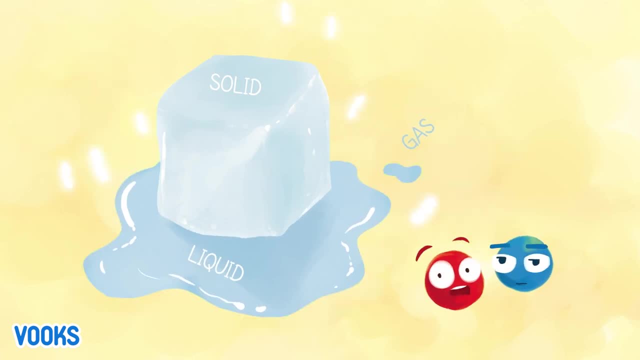 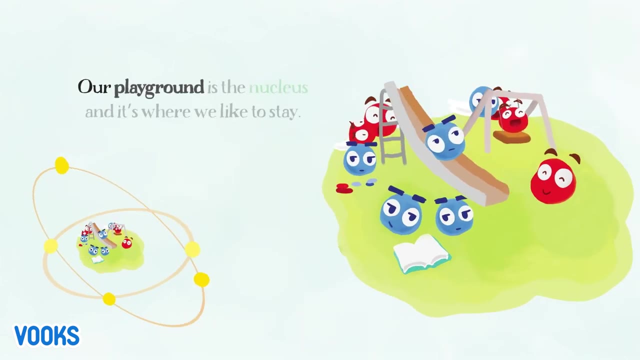 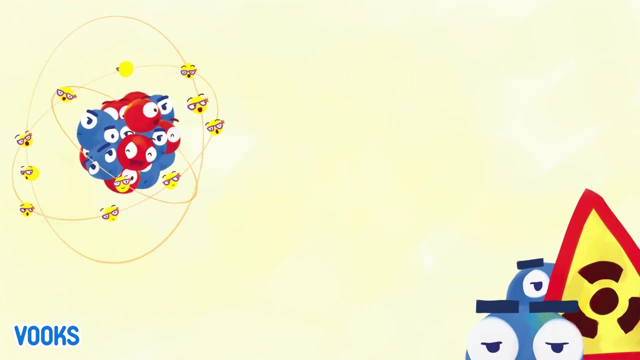 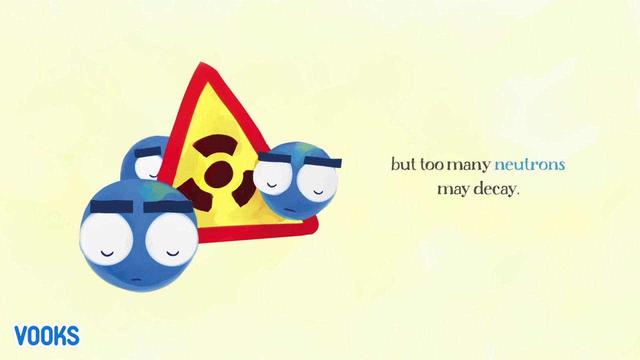 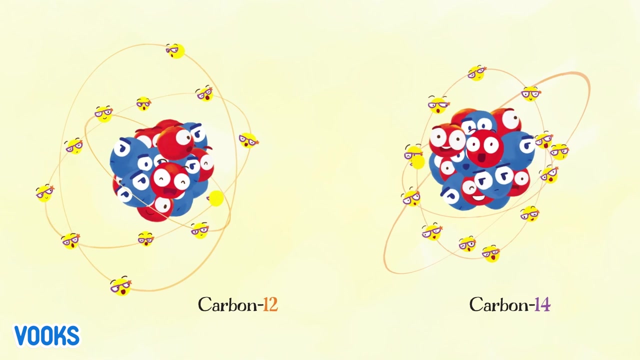 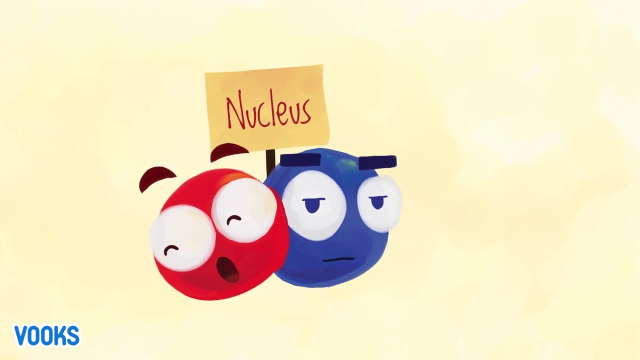 Solid liquid gas. Our playground is the nucleus And it's where we like to stay. Isotopes have extra neutrons, But too many neutrons may decay. Carbon 12. Carbon 14. Nucleus: The strong force keeps us stuck like glue. 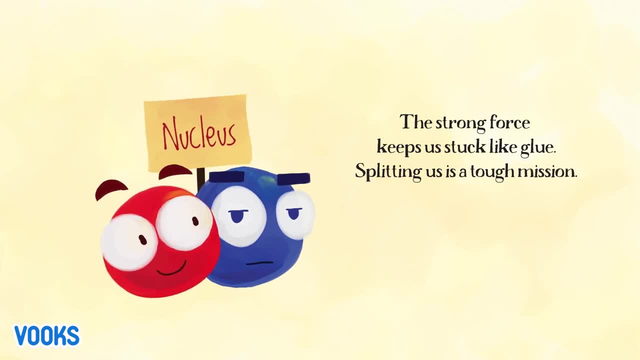 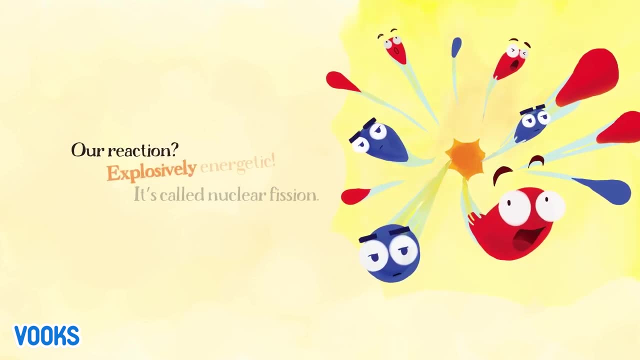 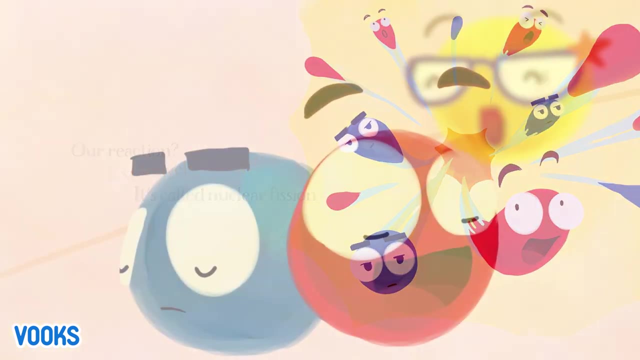 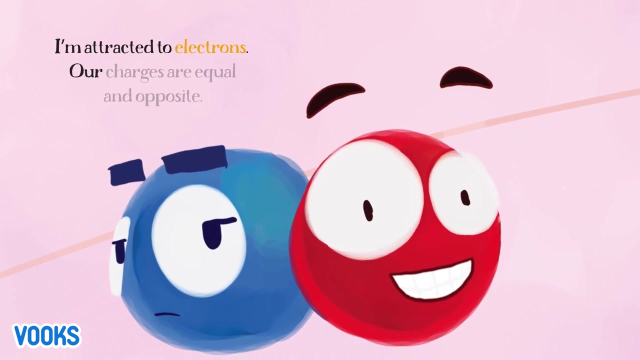 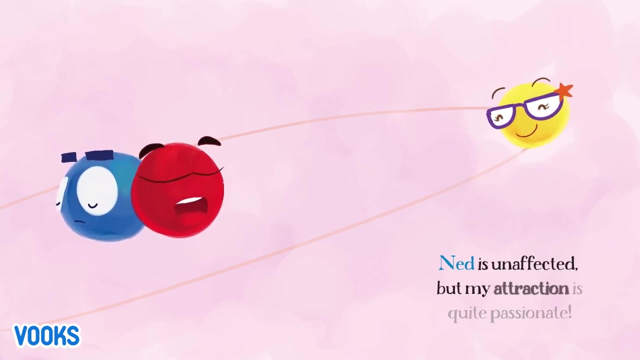 Splitting us is a tough mission. Our reaction: Explosively energetic. It's called nuclear fission. I'm attracted to electrons. Our charges are equal and opposite Ned is unaffected. But my attraction is quite passionate: BFF, Best friends forever. 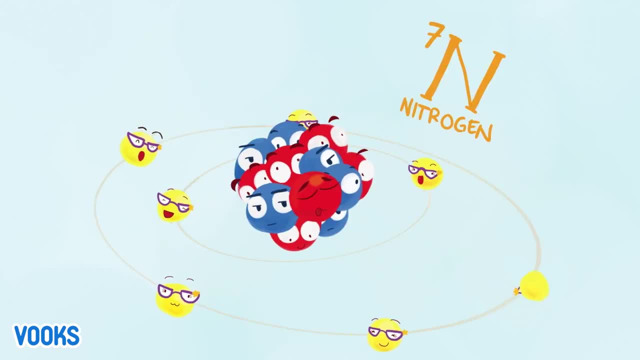 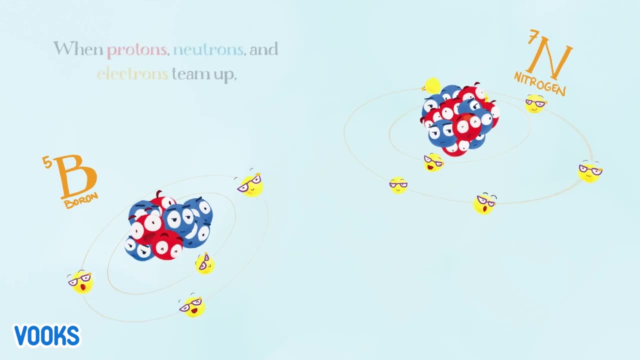 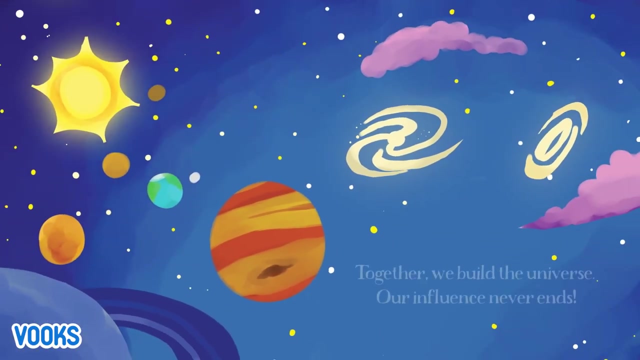 B, boron, N, nitrogen. When protons, neutrons and electrons team up, we are the best of friends Planets. We take part in the три�енты. Together, we build the universe On foot. 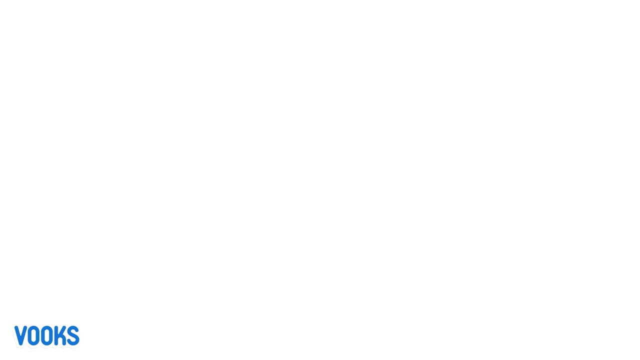 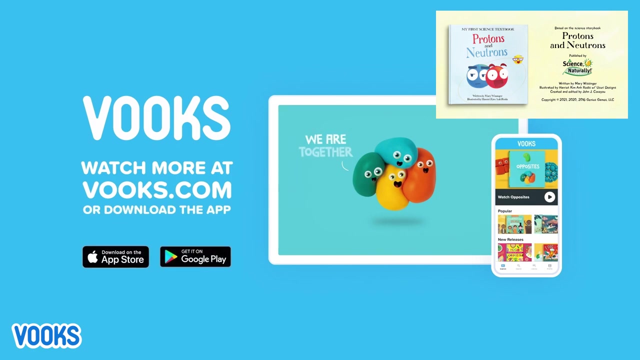 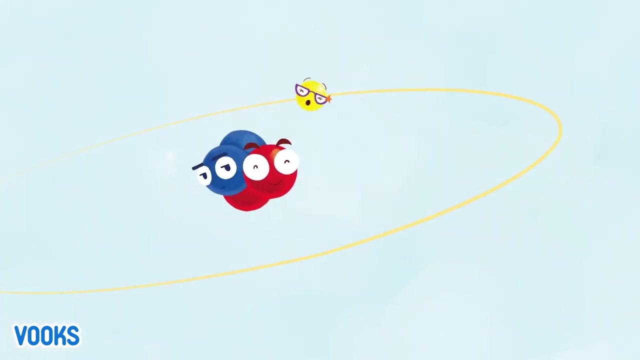 Together we join forces. We help you change the its UNום. Together we build the universe. Our influence never ends. Join us at lookscom Or download the app. My first science textbook: Electrons. I'm Ellie the Electron. 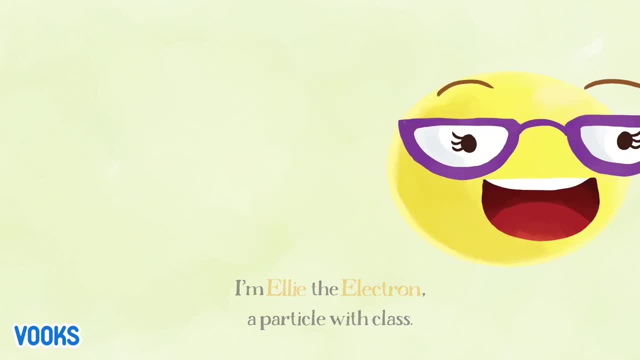 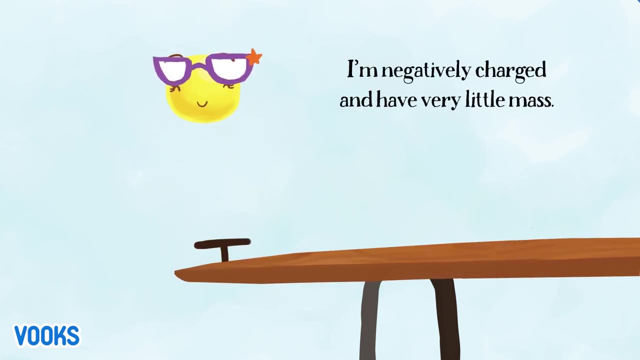 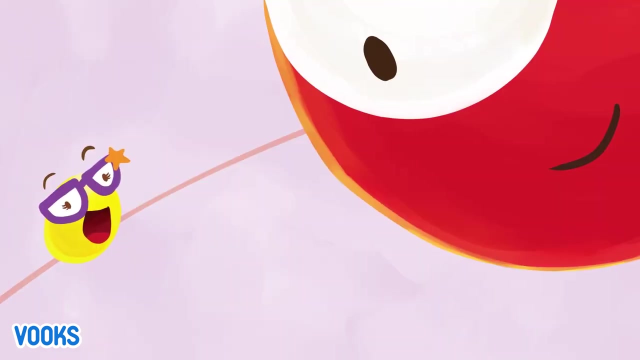 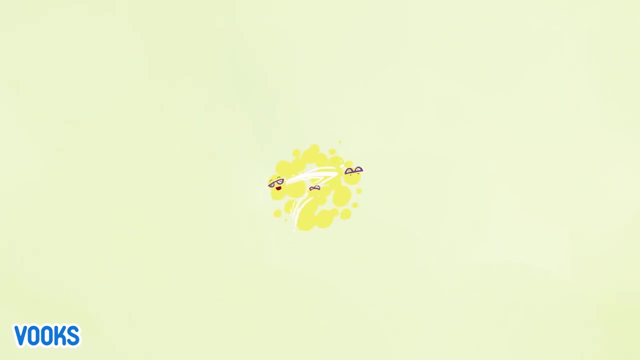 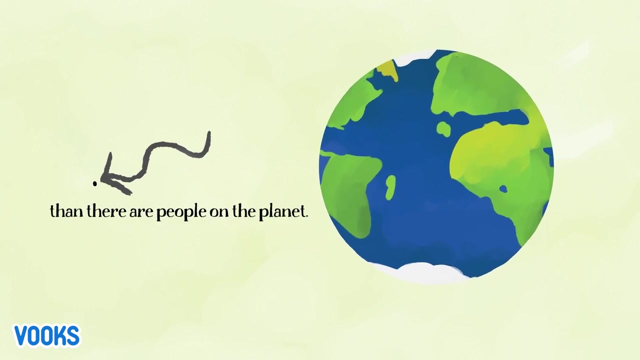 A particle with class. I'm negatively charged and have very little mass. I'm attracted to the proton. I'm almost 2,000 times smaller than it. More electrons could be produced. I don't fit on this dot, And there are people on the planet. 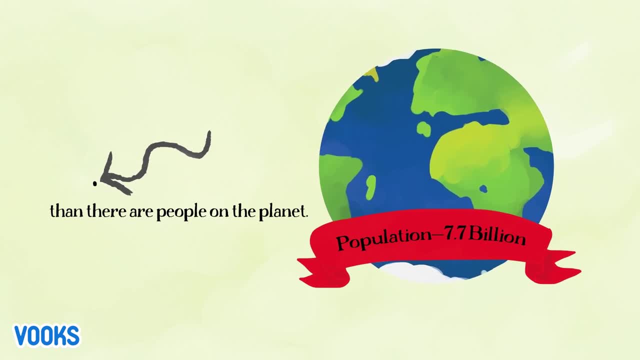 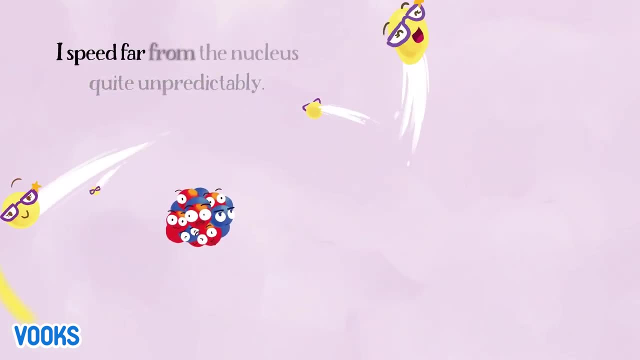 Population: 7.7 billion. I speed far from the nucleus, quite unpredictably. I mostly fly around in a cloud of probability. Pick which you'd like to calculate: My speed or my location? You can't know both at once. 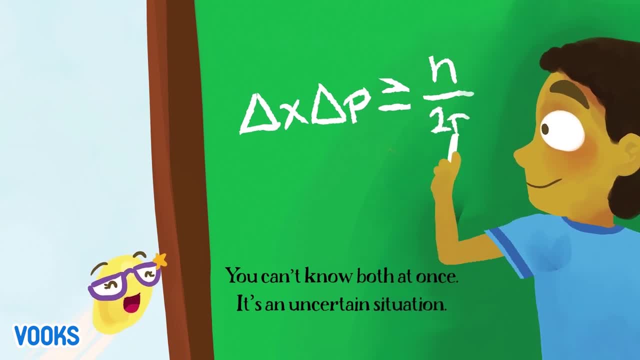 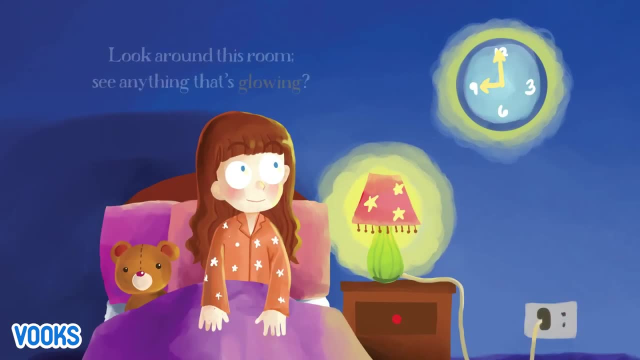 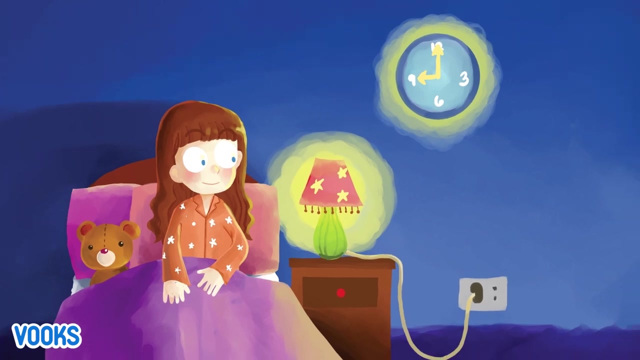 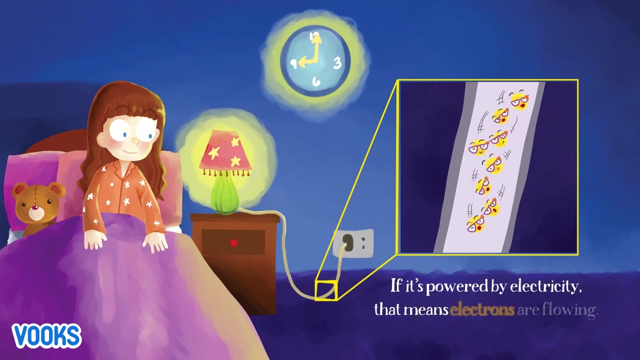 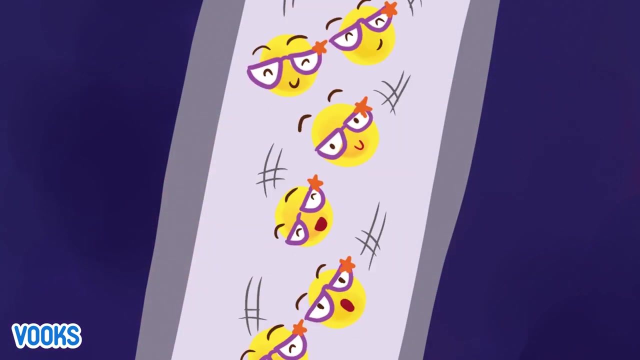 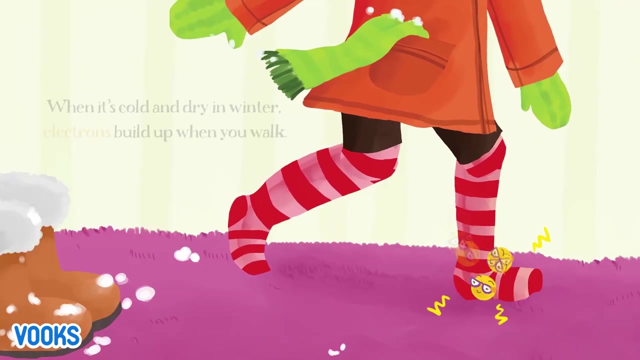 It's an uncertain situation. Heisenberg Uncertainty Principle: Look around this room. See anything that's glowing. If it's powered by electricity, that means electrons are flowing Electrons. When it's cold and dry in winter, Electrons. 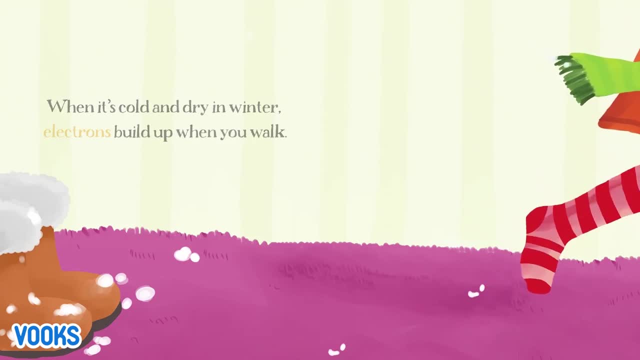 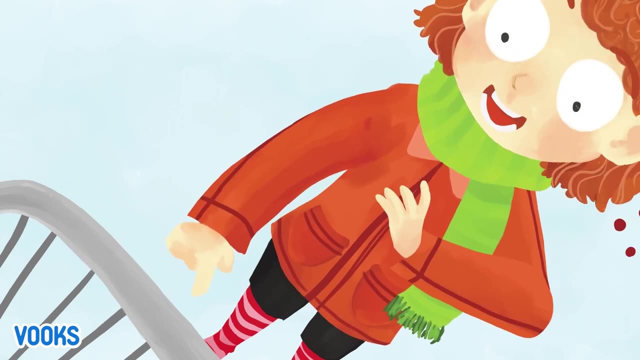 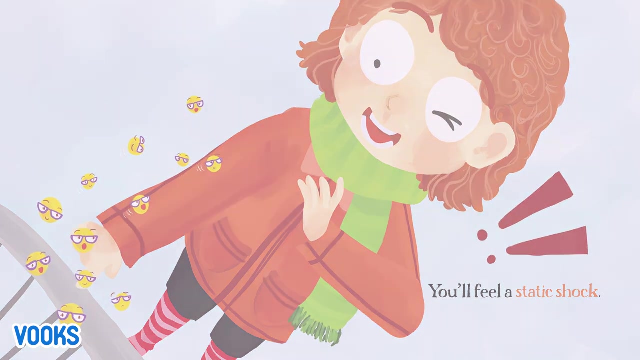 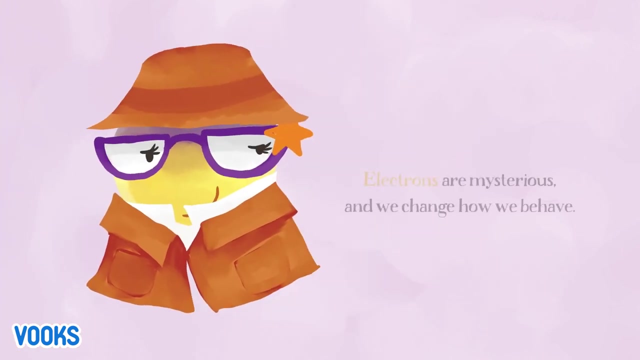 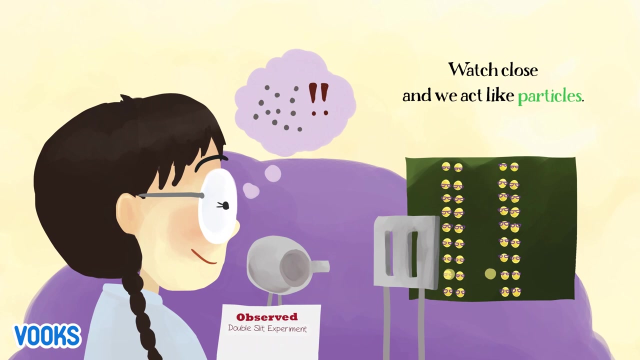 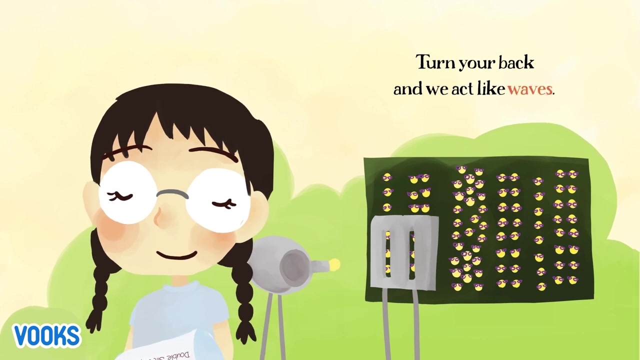 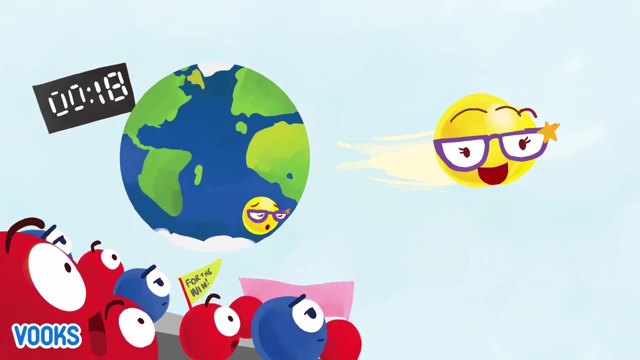 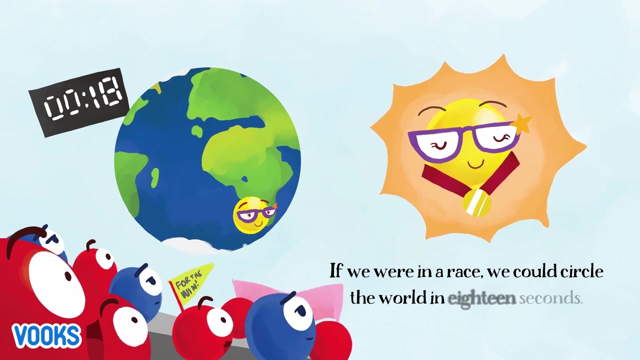 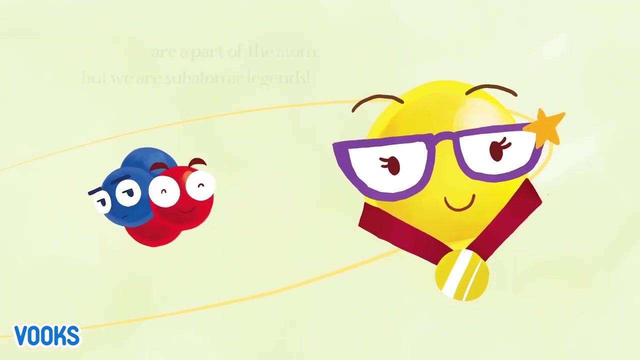 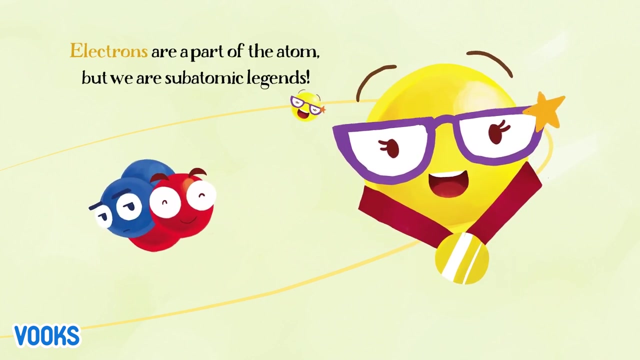 Electrons build up when you walk, Touch something and I'll jump to balance out. You'll feel a static shock. Electrons are mysterious and we change how we behave. You'll feel a static shock. Electrons are a part of the atom, but we are the atomic legend. 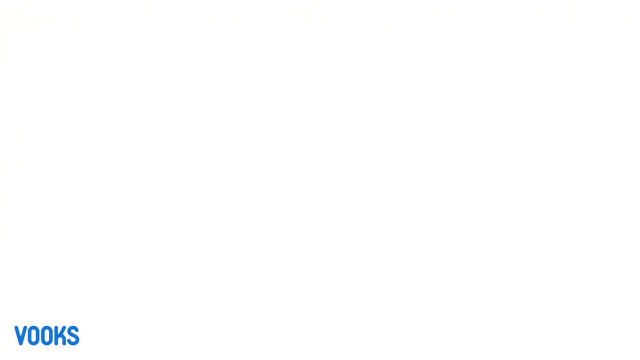 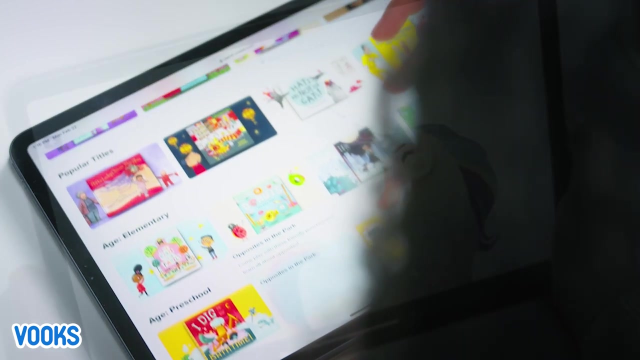 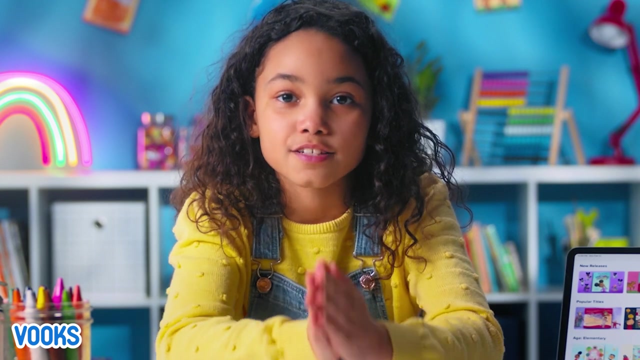 If you don't have books, what are you waiting for? It's a KidSafe ad-free library Full of so many storybooks that are brought to life. Ask your grown-up and start exploring more fun stories like these. You have to go and ask for books. 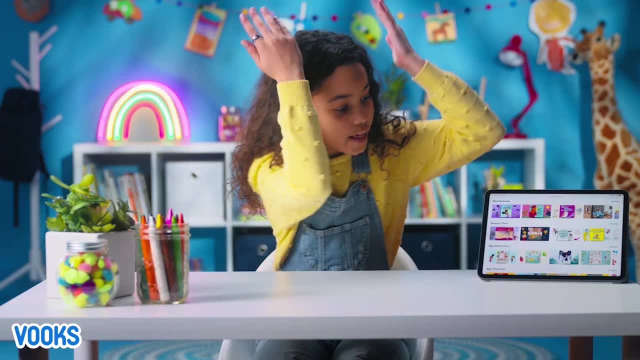 Enjoy the specialties of this app right here. Go on, Come on, Go off.